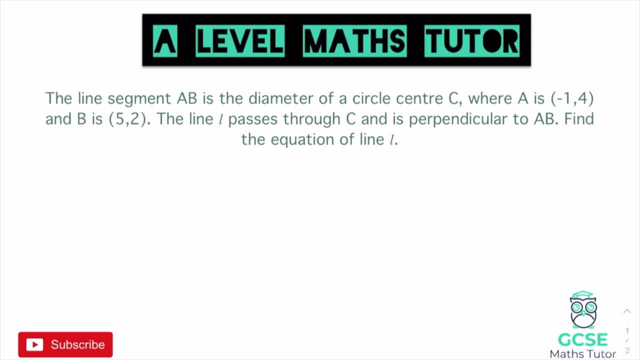 of this a little bit better. So to find the midpoint you take the coordinates and add them together and divide it by 2.. So if we focus first on the X coordinate to get the midpoint of the X coordinate, we would do 5 plus negative 1.. 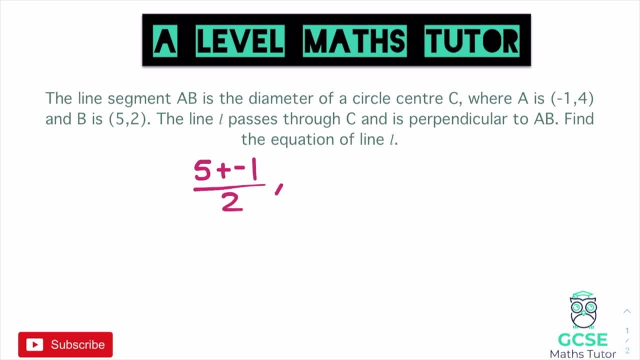 x coordinates and divide that by 2, and the other coordinate would be 2 plus 4, and again dividing that by 2.. So for that particular coordinate there, 5 add negative, 1 is 4, divided by 2 is 2, and 2 plus 4 is 6, divided by 2 is 3.. So we could probably draw an okay sort of sketch and think 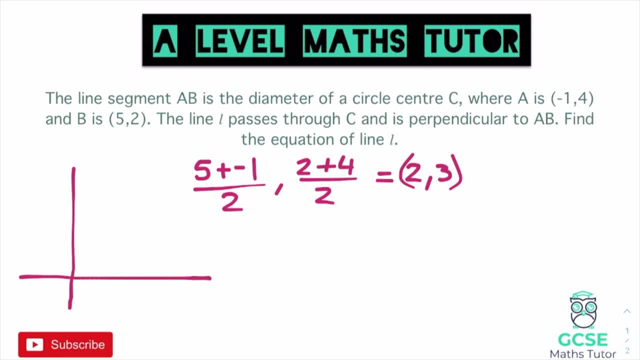 about what this looks like. So a is negative, 1, 4, so negative 1, 4. let's just imagine that's here. then our coordinate in the center is 2, 3, so that is to the right, obviously, and just a little bit lower than the 4. and then we've got another coordinate which is 5, 2, which is to the right. 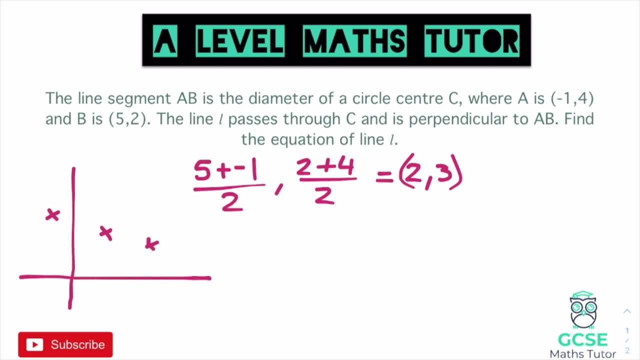 again and just a little bit lower. So it's going to look something like this: Now, obviously you're not going to be able to draw a perfect sketch of this, but you can just have something to help you visualize it. So if we imagine it looks something like that- although that wasn't very good, as my 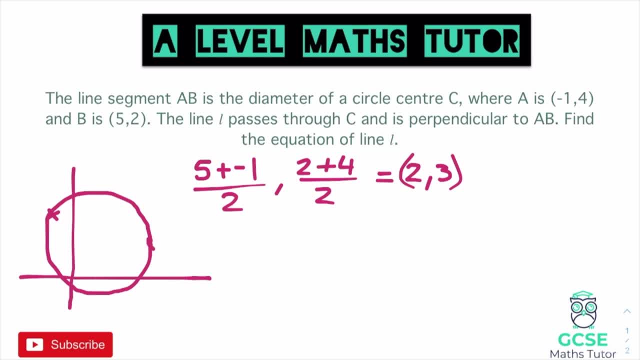 center doesn't look fantastic. so you can always get rid of these coordinates. and then we've got another coordinate which is 5: 2, and then we've got another coordinate which is 5: 2, and then we've got another coordinate which is 5: 2, and just put them back on so it suits your. 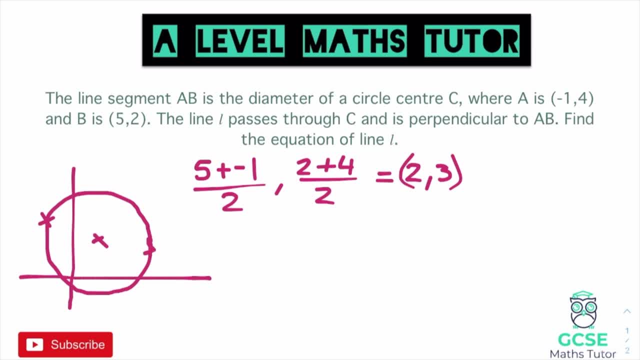 diagram. So let's say it's there, there and there. So now we have the coordinates of the center. So we could also draw in this line a, b and let's label that up. so that would be a and this would be b and we have our center point there and we are going to find the perpendicular bisector. 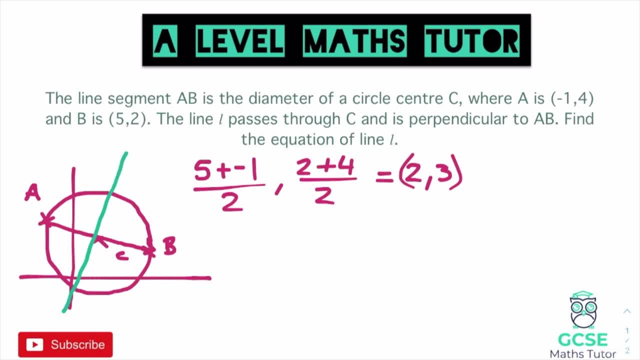 So if we find the or if we draw that in and imagine what it looks like, it's going to look something like that, and it'd probably be also worthwhile labeling on that center point, Denise. So how do we go about finding a perpendicular line? 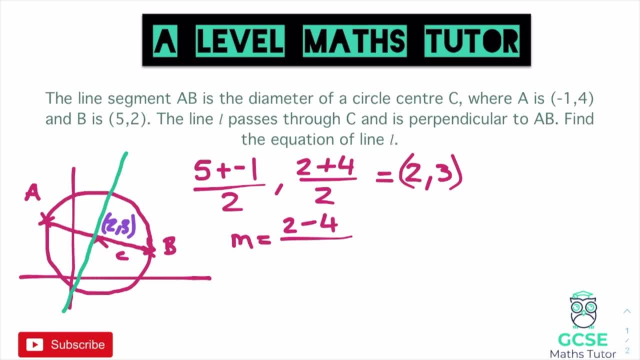 Denise. So how do we go about finding a perpendicular line? Well, first of all we want you to find the gradient. So we found the gradient of. well, then we can go about doing that to start with. So for finding the gradient, y2 minus y1, so that is going to be the y-coordinate of b. take away the y coordinat of 1,. 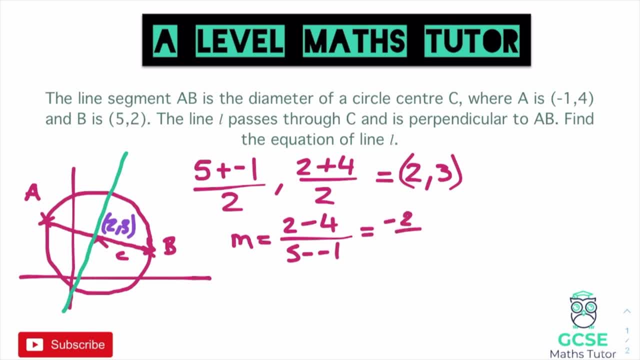 that comes out as negative two over six, which is minus a third. So our gradient of AB is minus one third, which means our perpendicular gradient is going to be our negative reciprocal and that comes out as positive three. So that is the first thing we need. 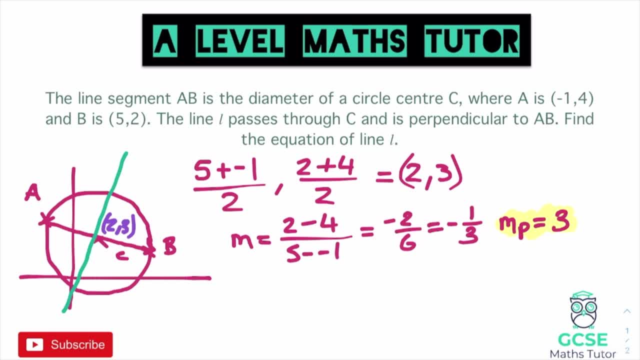 that is the gradient of our perpendicular bisector here. So now we can use our line equation: So Y minus Y one equals MX minus X one, And it is going to have to pass through that coordinate, through the centre which we can see here. two and three. 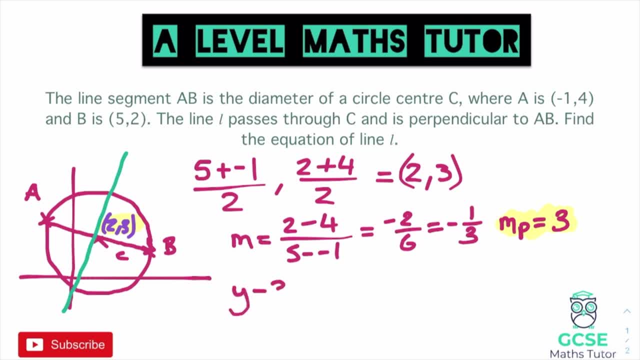 So we would have Y minus the Y coordinate of three is equal to M, which is three. I'm about to draw the bracket, let's get rid of that. Equals three lots of X minus the X coordinate, which is two. So if we expand that out, we get Y minus three. 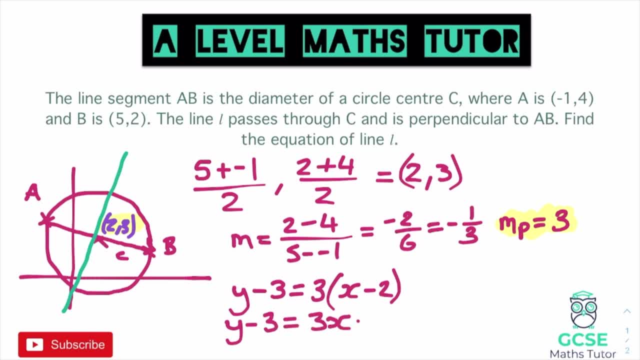 is equal to three X minus six. And then, of course, to finish this off, we want it just to say: Y equals, so add three to both sides. There we go, And we get: Y is equal to three X minus three, And that is the final line equation. 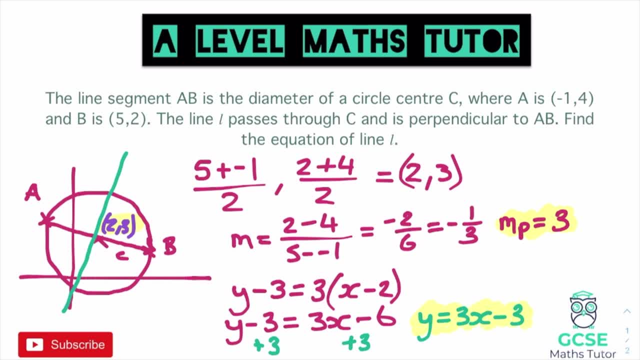 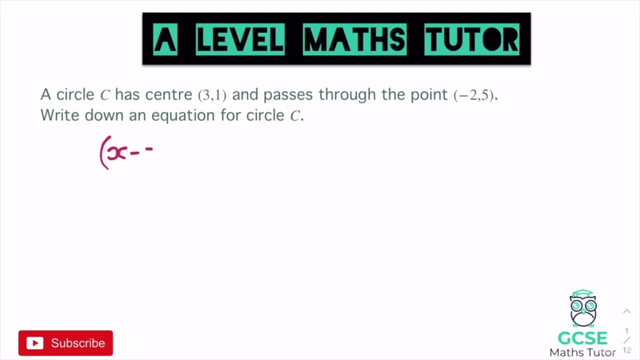 and that is the equation of our perpendicular bisector passing through the midpoint of AB, In terms of actually the equation of the circle. I'm always just going to write that down. So I've got X minus A, which is the first coordinate. 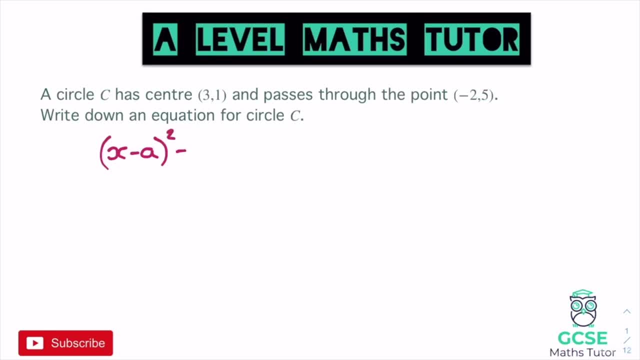 or the X coordinate within the centre squared. Add to that Y minus B, which is obviously the Y coordinate of the centre squared, And that's going to equal the radius squared. So if we plug these numbers in that we've been given three and one. 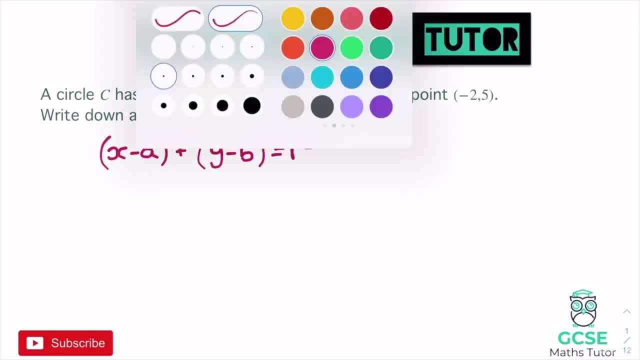 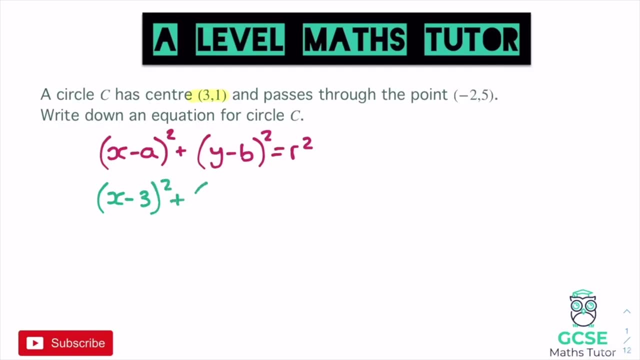 let's just put them into the equation and see what we get. So there we go. We've got X minus three squared. add Y minus one squared and that is equal to the radius squared. I'm going to do this in two different ways. 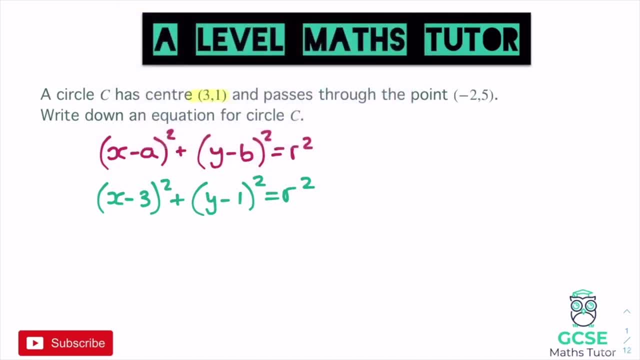 So if you've seen this before, you might have only used one of the ways, so I'm going to show you the both. but in terms of what we did in a GCSE, maybe at this point we'd have imagined these two coordinates okay. so if I imagine the point three, one which is the center, it 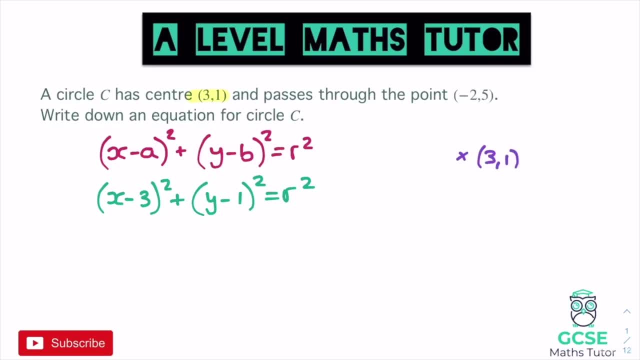 does always help if you can draw a little diagram of these. but if we imagine three ones, the center and then negative two five, let's have a. just have a little think. it probably looks something like this: there we go and negative two five is somewhere over here. let's have a think. negative two fives. 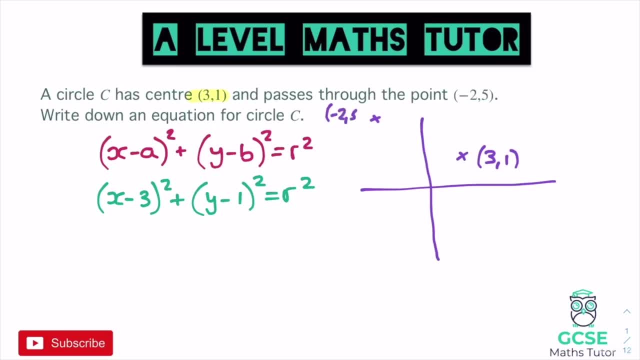 maybe over there, somewhere. there we go. but in terms of looking at these two points, we would find the length of the radius by using Pythagoras, like we've just talked about, and we would look at the base or the, or the rise and the run there, or the change in X and the change in Y, and then we just use Pythagoras to 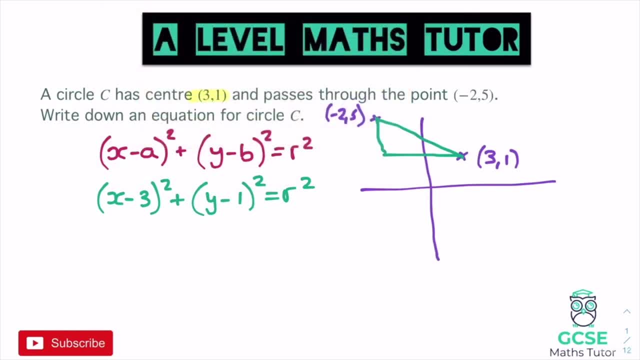 work out the radius. so in terms of the base length it goes from negative two on the left there over to three, which is a length of five, and going up it goes from one up to five, which is a length of four. so you can use Pythagoras to work out. 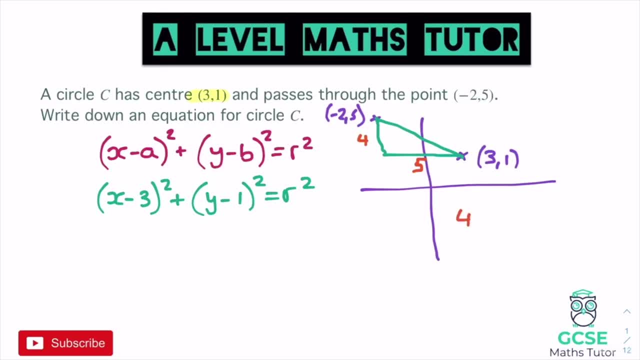 the length of the radius there and we can just do that quite nice and easy. we can do four squared plus five squared, which is 16 plus 25, which is 41, and then you can just square root that for the radius. so R equals the square root of 41. there we go, but obviously we want to. 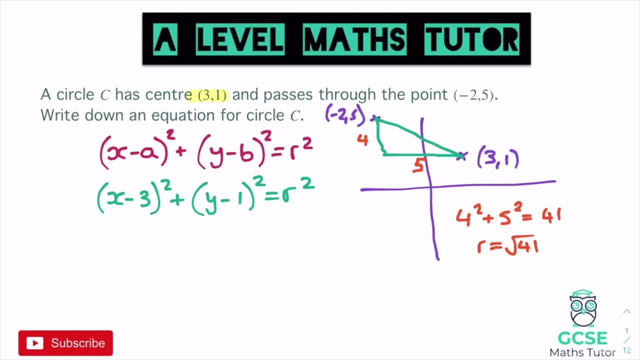 know what the radius squared is. so when it's in nice little square root like that, we can just take away the square root and it'd be 41, so we could finish off our equation here. it'd be X minus three squared plus Y minus one squared. 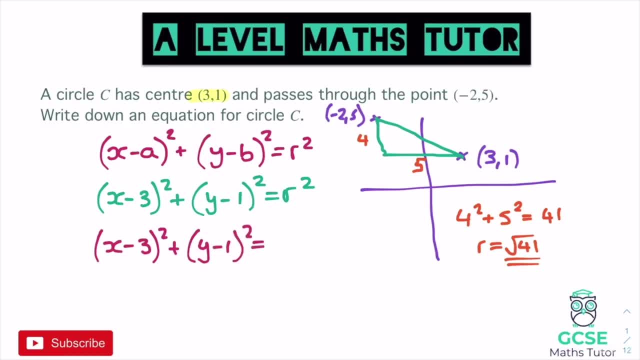 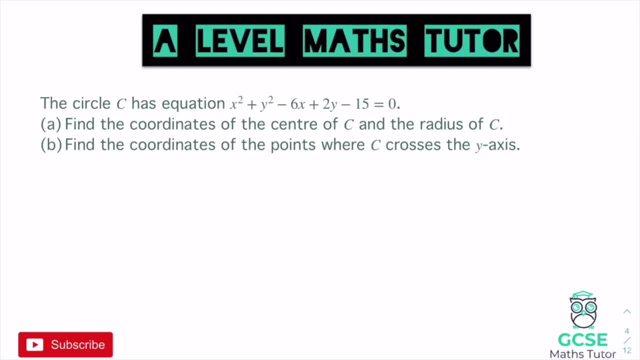 equals the radius squared. the radius is root 41, so 41. so it says the circle C has equation. and then we have the equation here and lots of pieces. we've got X squared, Y squared, X, Y's and a number and it all equals zero. so let's find the. 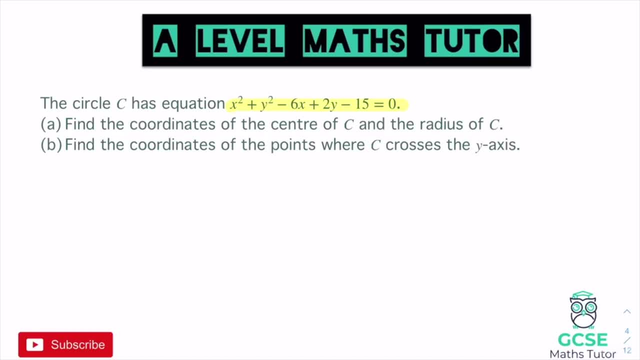 coordinates of the center of C and the radius of C. and then we've got another question here that says: find the coordinates of the points where C crosses the y-axis. so I'll have a look at that in a sec. but this actual equation here has to be rearranged in order to get it into the format that we want of. 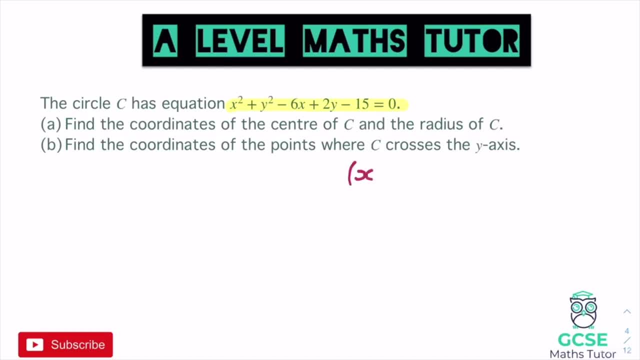 this thing. we know what the format looks like. we've got X minus a in brackets squared and then we've got Y minus B in brackets squared and that equals our squared. so we have to rearrange this. we need to get all those numbers on the right hand side and then we need to get these X parts into. 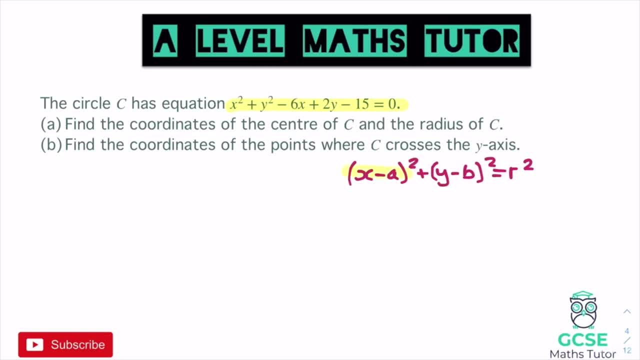 brackets and if you hopefully recognize this, you should recognize that this looks very similar to completed square form and this is where we're going to use a bit of completing the square to get it into this format. if we have a look at the pieces that we have in our equation, we've got some X pieces here. 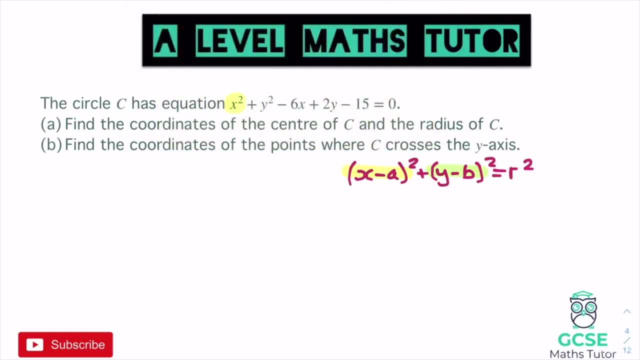 we've got, and I'll highlight this in that color: there we've got the X squared and we've got minus 6x. now, if we just forget about everything else there and we group those together, we'll have X squared minus 6x. okay, now, if we were to 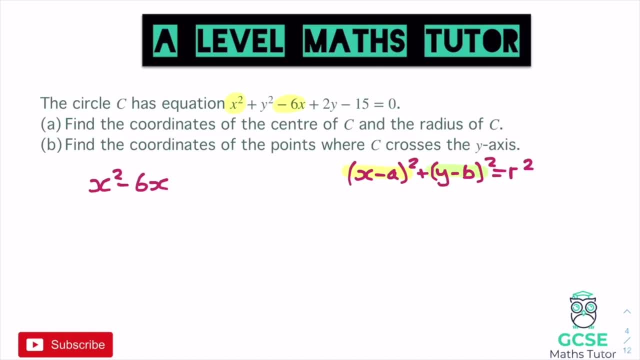 complete the square on that. okay, just on that part. there we would obviously half the coefficient of X, so it'd be X minus 3 in brackets squared. and obviously, if you're not sure I'm completing the square, don't forget I've linked that in the description below. so check that out first and then obviously we need to get. 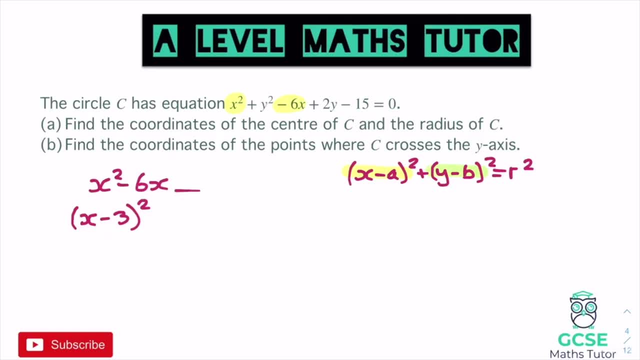 that back to zero because there's no number after this. so to get that back to zero, thinking about what that would expand to, while negative 3 times negative 3 would give us positive 9, so I'd also have to take away 9 and that obviously. 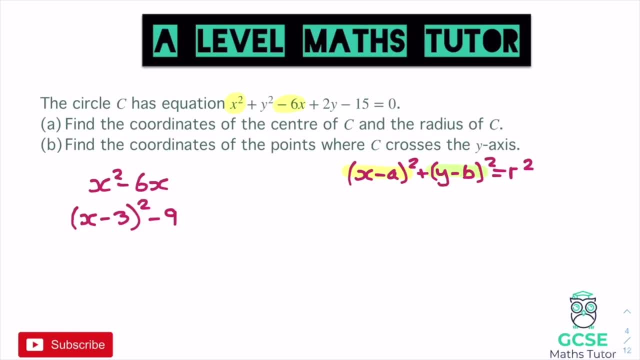 that expression there would give us X squared minus 6x, sometimes just writing that in completed square form. we also have the Y pieces. now if we have a look at the Y pieces in there, let's just highlight those. we've got Y squared and a plus 2y. now if I put those in, we've got so. 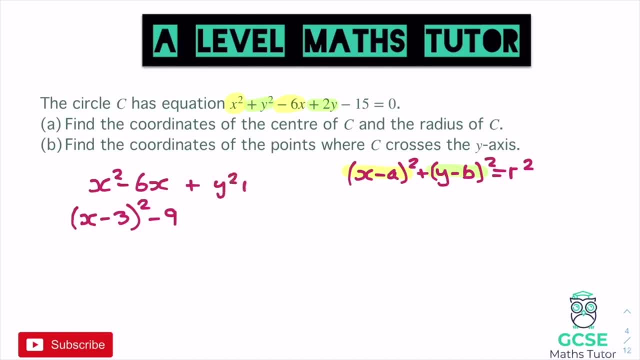 I'll put a plus here as well. we've got Y squared plus 2y. now, if I complete the square just on that and let's keep the plus there as well, we would have the coefficient of Y, so I'd get Y plus 1 there. we go in brackets squared when we 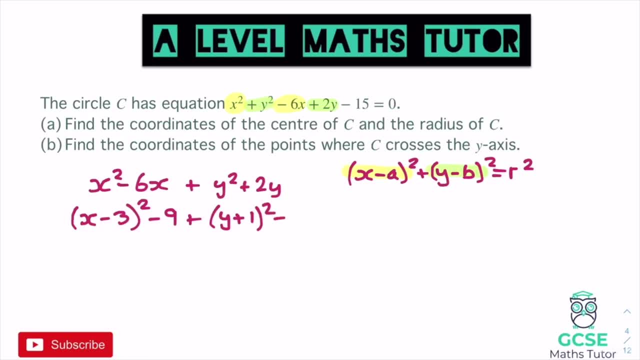 expand that that gives us plus 1. so we have to take that one away to make it balanced to the expression above the Y squared plus 2y, and that would obviously complete the square on that part. so so far what we've done, we've completed the square there. that's given us a little bit below and we completed. 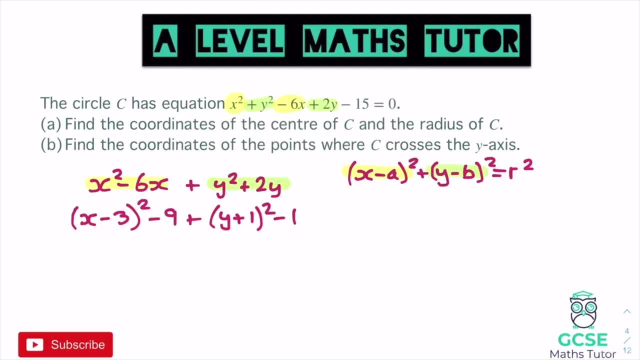 the square will have six parts there and again for that bit below as well. then we've still got that minus 15, so we need to bring that minus 15 back in. there we go, and it all equals zero. so as add the minus 15 in, there we go and that all. 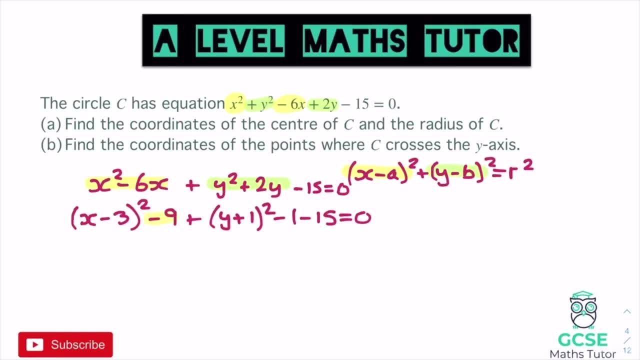 equals 0. now if we have a look at just the numbers that we've got there, we've got a minus 9, a minus 1 and a minus 15. now if I group those all together- and I'll probably skip a few steps on the next question here- but if I group all- 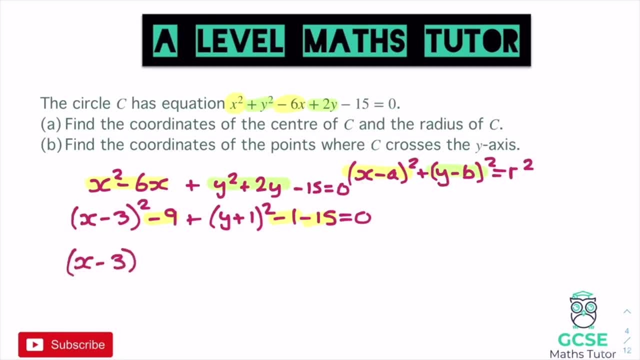 the numbers together and I put them all at the end. let's see what we've got in brackets squared plus the y, plus 1 in brackets squared, and then all of those numbers we've got minus 9 minus 1, that's minus 10. minus another 15 is minus 25. there we go, that all equals 0. 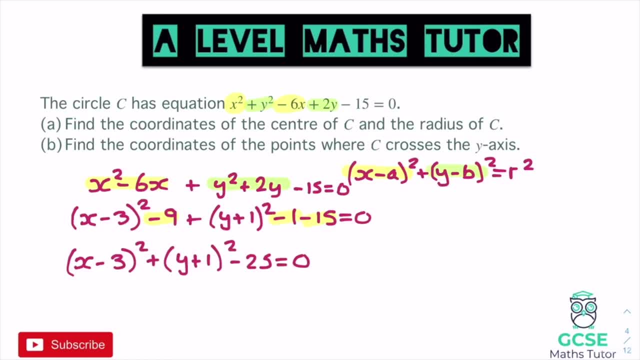 obviously, just to finish this off, we just need to move that 25 over to the other side now, get it into the equation of a circle, the format that we've looked at throughout the video. so if we plus 25 to the other side, just to finish this off, and then we can get the center and the 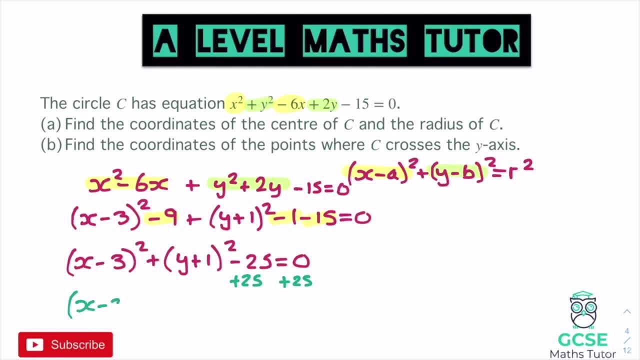 radius from that. so we've got x minus 3 in brackets squared, plus y plus 1 in brackets squared, and that equals 25. now, from there we can get the coordinates of the center and we can also get the radius. now the easiest part there. well, I think they're both relatively simple once you've got. 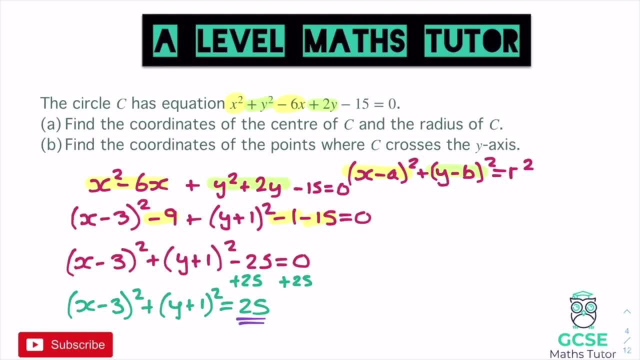 to this point. but it's nice and easy just to square root this number at the end to get the radius. so we know that the radius is going to equal the square root of 25. as that is, r squared at the end equals the square root of 25 and in this case that becomes a whole number, that becomes 5. 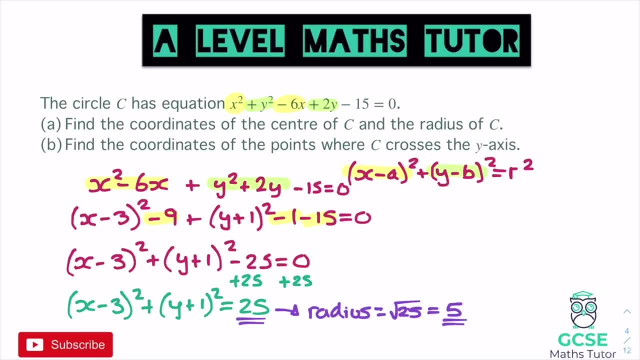 okay, obviously the square root of a number is positive and negative, but we can't have a negative radius, so it's just going to be 5 there for the length of the radius. now, in terms of actually getting the equation of- sorry, the coordinates for the center, now, obviously we 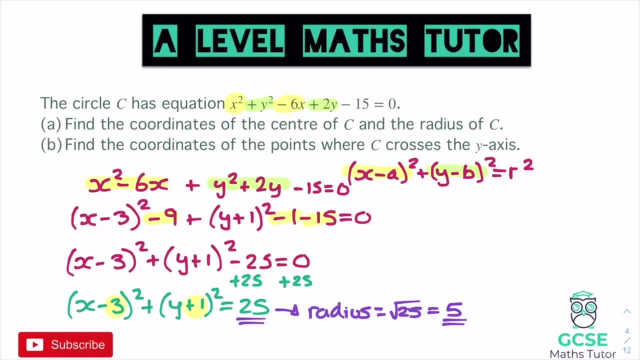 know it's minus a and minus b on these parts here, so a is going to have to be that 3 right there. so the center, there we go and we've taken away 3, and on this one here we just need to be a little bit more careful, because 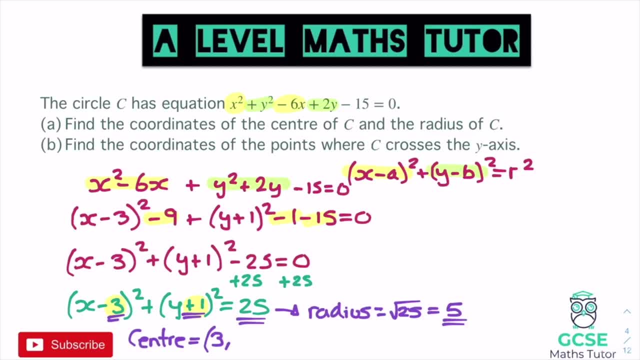 we've got a plus 1 there, so we must have taken away negative 1 in order for it to turn into positive 1. and there we go. that's our radius and our center, taken from that equation. okay, so there's our two key parts for part a. we've got our radius, which is 5, and our center, which is 3 and minus 1. 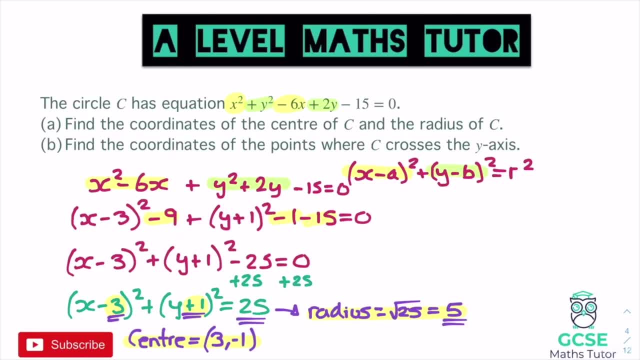 just need to be careful there. when there is a positive number in the bracket, like the y plus 1 that you remember, therefore it must have been negative 1 that we took away in order for it to become positive now. the second part here says: find the coordinates of the points where c and y are. 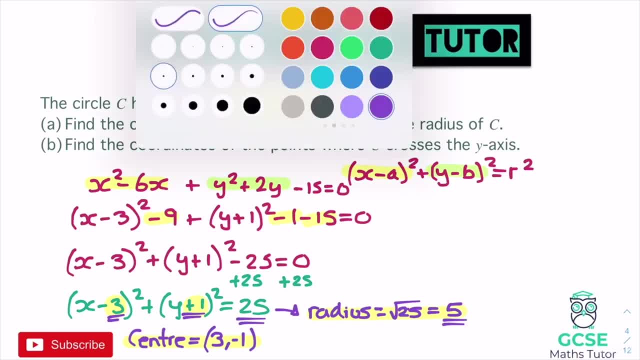 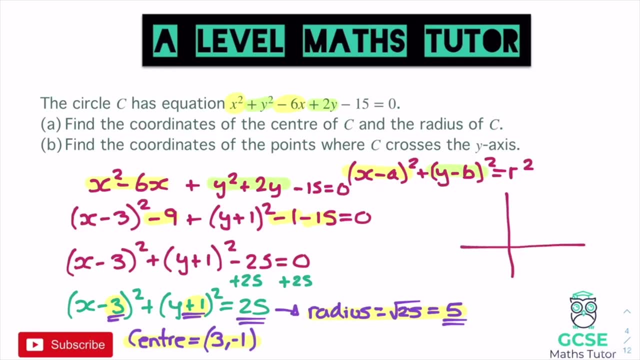 equal to the points where c crosses the y-axis. now, in terms of actually thinking about this logically, in terms of a coordinate graph, if we had a circle, let's think about what this would look like. let's have a think. the center is at 3 minus 1, which is somewhere there, and if i was to draw a 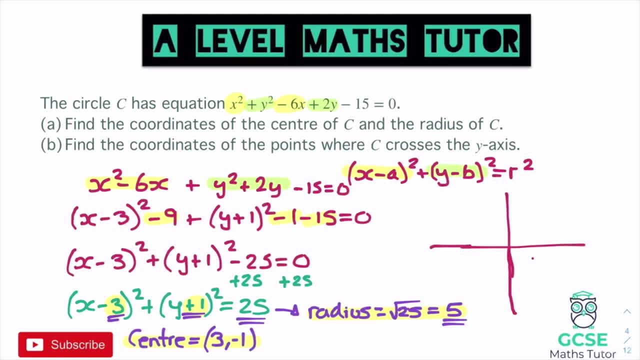 circle in which i always don't really like doing on the screen here because it's not the easiest to draw, but it would look something and it's a really rubbish circle. but there we go. it looks something like that if i was to draw a basic sketch. let's get rid of that center point, because that really 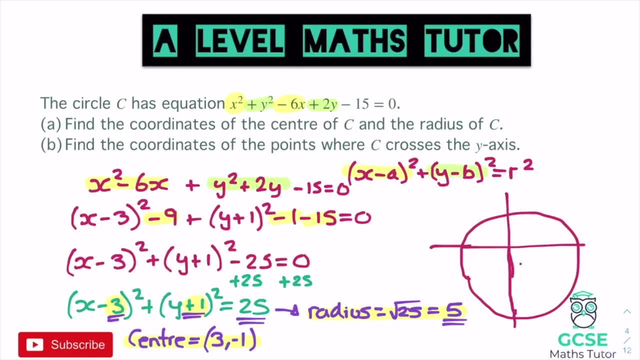 does not make it look good, there we go. let's imagine that we've got a circle and we've got a circle in the center. there we go. 3 minus 1, not not to scale, but there we go. we have these two coordinate points where it crosses through the axes. so here and here. now the logical thing about. 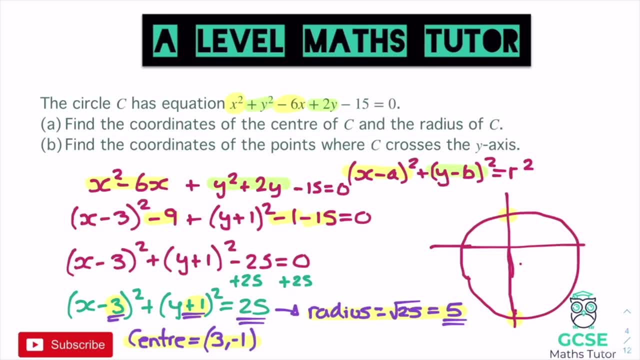 this question is that any point on the y-axis there the x coordinate down here- is always going to be zero. so effectively, if we want to know where what the y coordinates are, where it crosses through the y-axis, all we have to do is sub in: x equals zero. let's get rid of that sketch there. 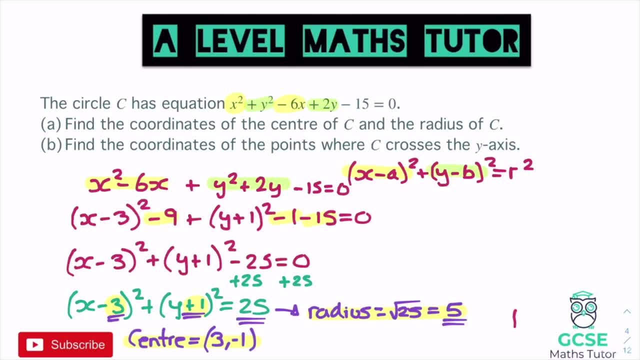 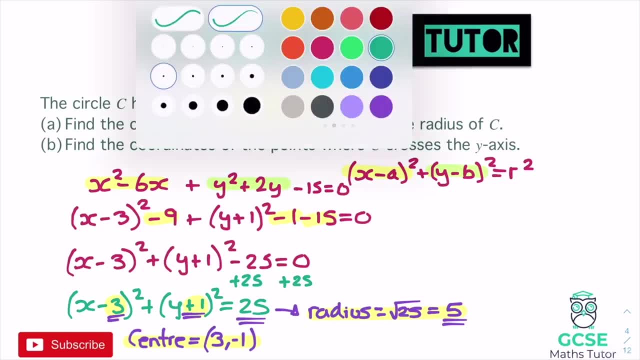 because it's a little bit of an embarrassing sketch. there we go, but just to give you a sort of an idea as to what we're actually looking at, we're looking at when x equals zero. so if i sub that into my equation, my equations there, i just want to know: what does it equal when? 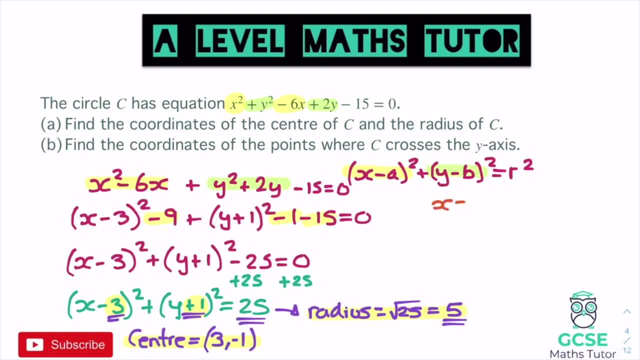 x equals zero. let's put that in. so when x equals zero, what do we get? and i'm subbing it into this equation just here: so we get 0 minus 3 in the first bracket. so we get negative 3 squared plus. we don't know the y coordinates. so we've got y plus 1 squared and that equals 25.. 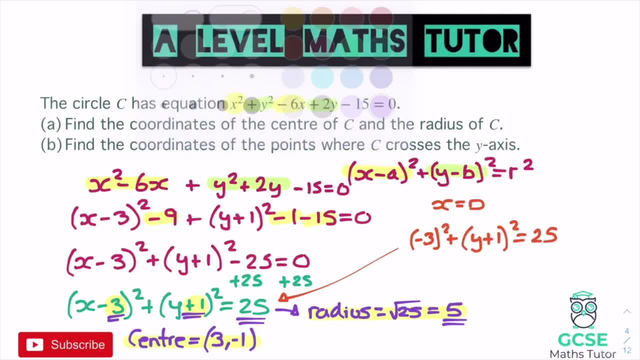 so we just need to rearrange this and our negative 3 squared is 9. so actually i could just think that that's 9 there, and if i take away 9 from both sides, we get y plus 1 in brackets squared equals 16 when you take away that 9.. now if i square root both, 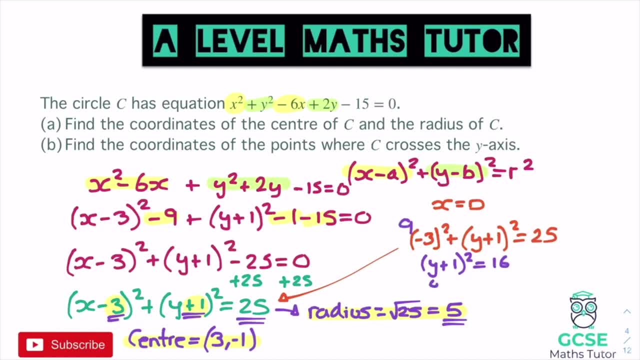 sides. obviously we want to get y, find out what y is. so square root both sides, we get y plus 1 equals this plus and minus the square root of 16, so it could be plus and minus 4.. and obviously then we just need to take away 1 from both sides and we get y equals. 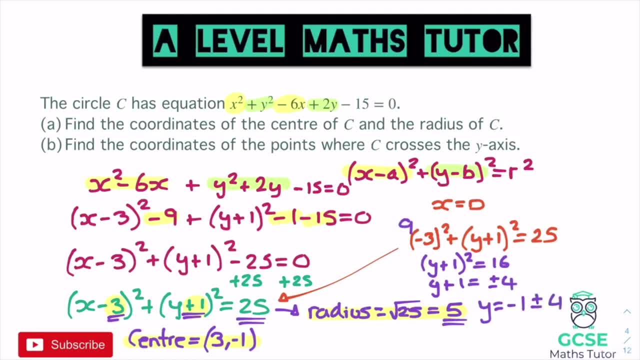 1 plus and minus 4, and that there will give us two values. okay, because you could have negative 1, add 4, so y could equal 3, or we could have negative 1, take away 4, which would equal negative 5.. so we've got 3 or minus 5 in terms of where it crosses the y-axis. they are the two coordinates. 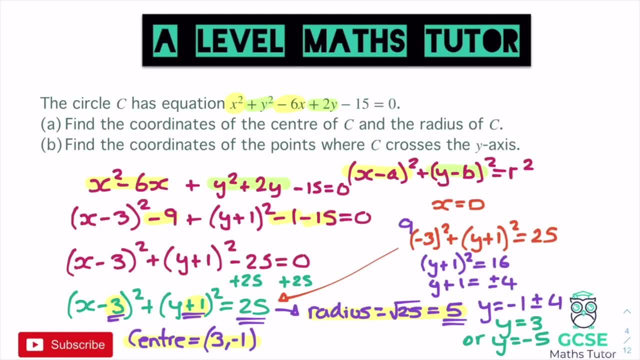 there. so obviously you could draw a bit more of an accurate sketch. now you know where it crosses through the y-axis. but there we go. that's how we're going to go about solving these two parts of the question. so for this question, look at this equation that wecould do is we will be taking a score of 4 and we will be putting 1 and 2 in the bottom row. 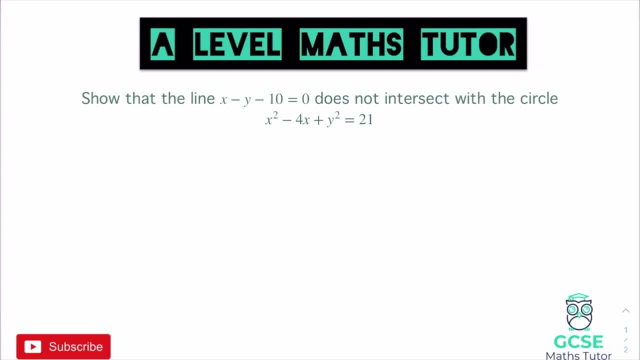 at intersecting circles with lines. it says: show that the line x minus y minus 10 equals zero, does not intersect with the circle. and then we have our circle equation. So we've got our two pieces and obviously the process to solve this will be using simultaneous equations. 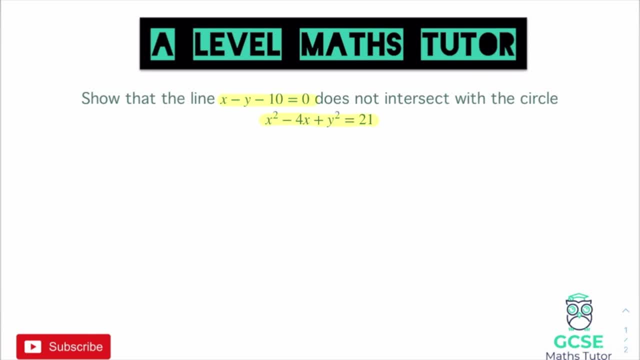 So although we looked at quadratic simultaneous equations before, this question is slightly different. as it says, this fact here does not intersect And obviously in this relation we are actually looking at the actual circle. So the process to do this is substituting that first equation in, So we want to make that x or y equals. Now look at your circle. 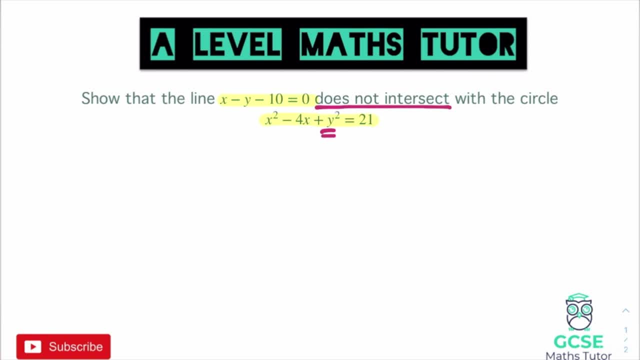 equation, because there are two x's in that equation but there's only this one y-squared piece. So it would be easier for us if we could make it say y equals. So if we take our first equation and add y to the other side, we get x minus 10, which is equal to. 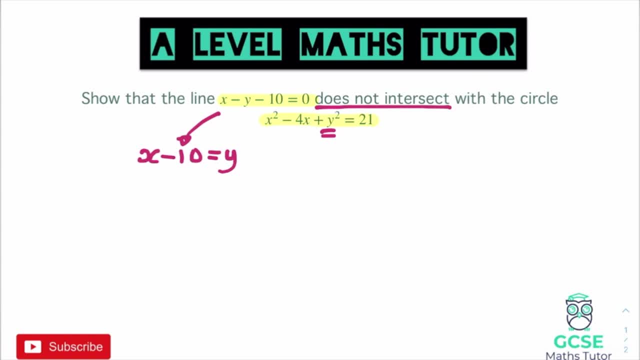 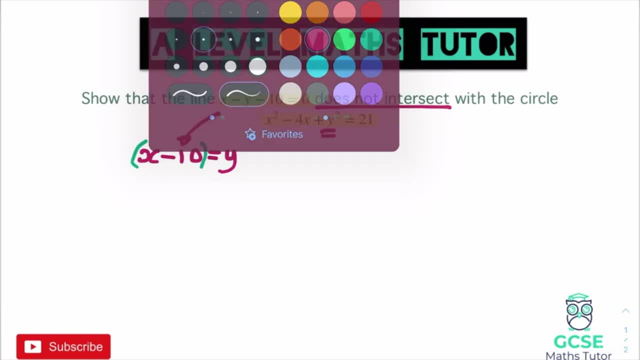 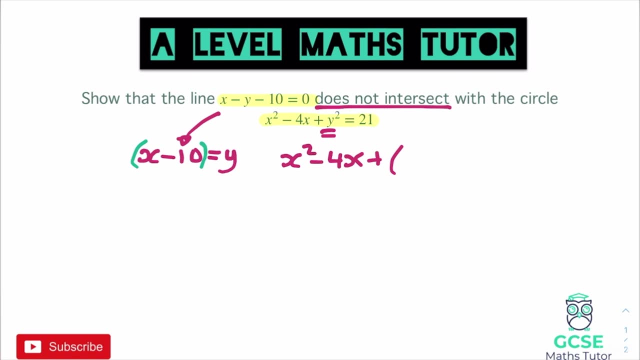 y, Of course you could write that as y equals x minus 10.. So if we take that and substitute and substitute, substitute it into our circle equation, just put in a bracket around x minus 10.. When we substitute that in, we get x squared minus 4x plus and then we have our x minus 10, which is going to be: 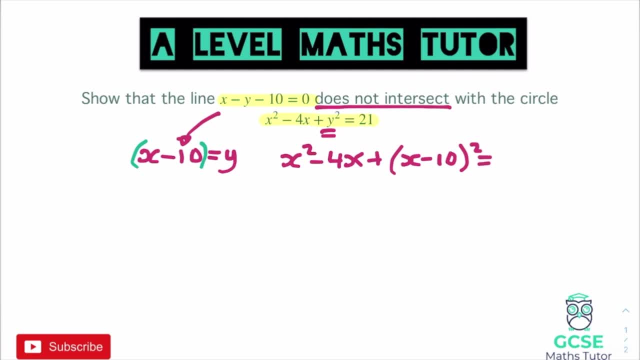 squared And that is equal to 21.. So now we have an equation that is going to be a quadratic that we're going to need to make equal to 0. And then to show that it doesn't intersect, we're going to have to show that it has no real roots. So, having a look at this, then let's first expand that double. 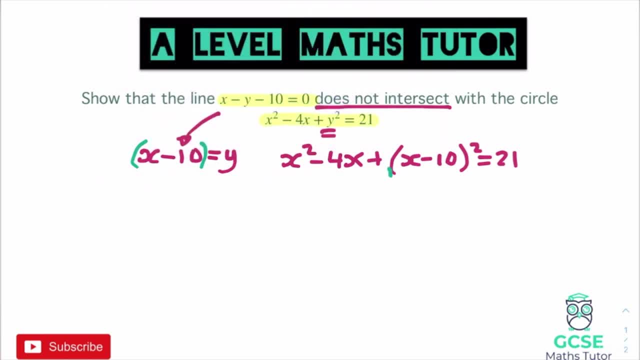 bracket And obviously, if you are quick at expanding your double brackets, you can obviously just write the answer to that, which is x squared minus 20x plus 100.. So if we write that all out and simplify it, we've got 2x squared. so 2x squared, We've got a minus 4x minus 20x, which is: 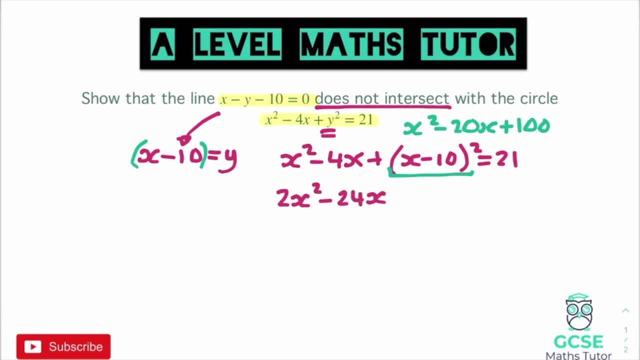 going to be minus 24x. We have a plus 100 at the end of the equation, so we've got a minus 24x, But we're also going to have to minus this 21 to make sure it equals 0. So we can simplify. 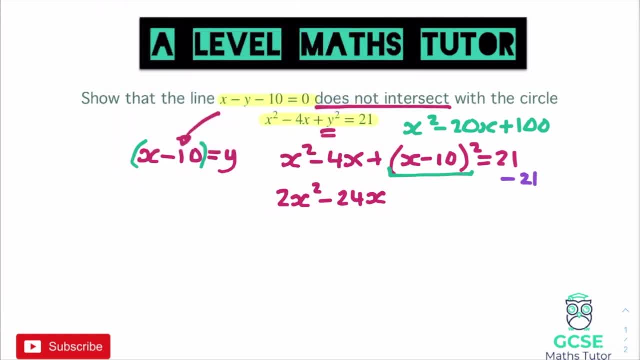 that straight away, which is 100, take away 21,, which is going to be plus 79. And that is now equal to 0.. Now, obviously, if they did intersect at this point, we would want to solve this equation. We would want to find our x coordinates and then we would substitute them back in to find 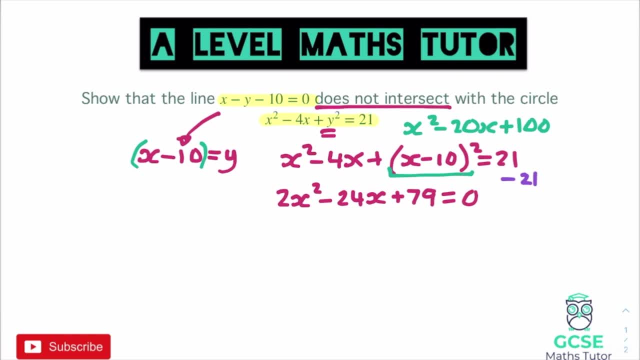 our y coordinates, But this says does not intersect, so we will look at the discriminant. We are going to look at b squared minus 4ac and then identify our a, b and c. So a is 2, b is. 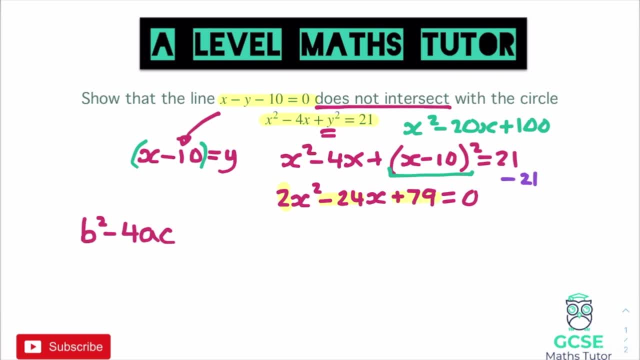 negative 24, and c is 79.. And again, it's always worth writing them down: a is equal to 2,, b is equal to negative 24, and c is equal to 79.. OK, so putting that into b squared minus 4ac, we are. 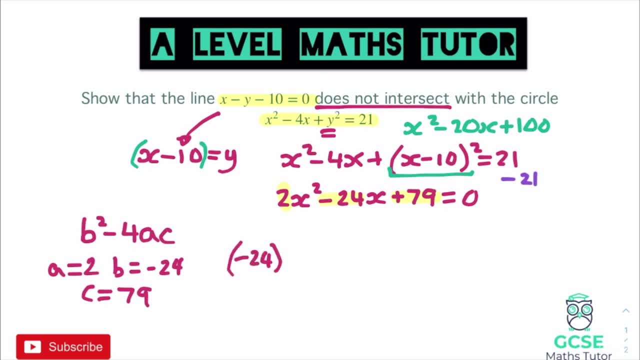 going to have negative 24 squared and take away 4 times 4. So we've got a minus 24 squared and 2 times 79. And if we type that into our calculator- and let's just type that in- 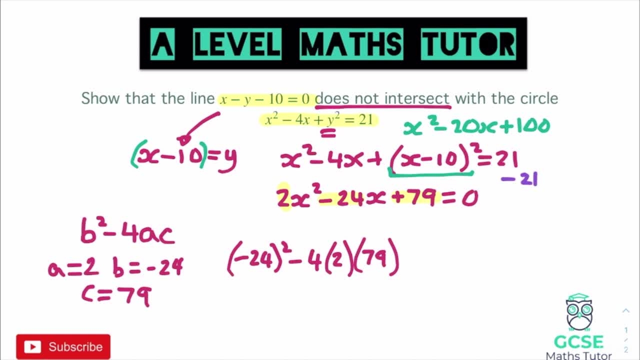 we get negative 24 squared minus 4 times 2, times 79. And the answer comes out as minus 56. So we know that when b squared minus 4ac is less than 0, that less than kind of looks a little bit. 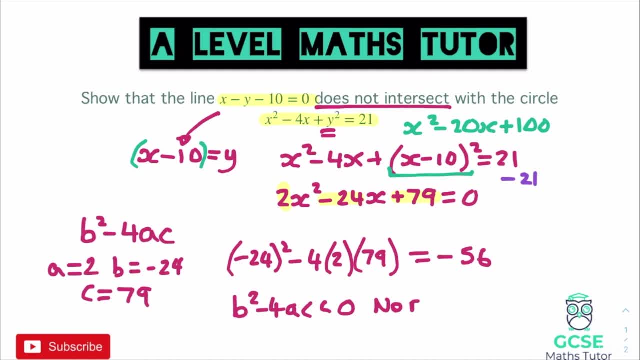 like my c there, but that means it has no real roots. OK, so because we've got an answer of negative 56, we have no real roots and therefore these do not intersect. OK, so when looking at tangents to circles, we just need to remember that the tangent 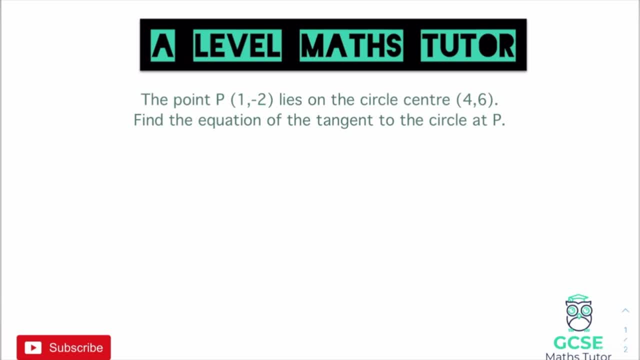 is going to be perpendicular to the radius. So for this question here, where it says the point p, which is 1 minus 2, that lies on the circle with a centre- 4, 6, and it wants us to find the equation. 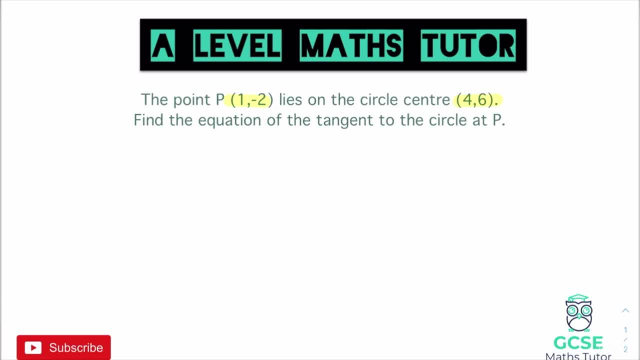 of the tangent to the circle. at that point we can start by finding the gradient of the radius. Now what you can do on a question like this is to draw a little diagram which might help you to visualise it, and that's fine to do as well. It says the centre of the circle is 4,, 6,, if we imagine. 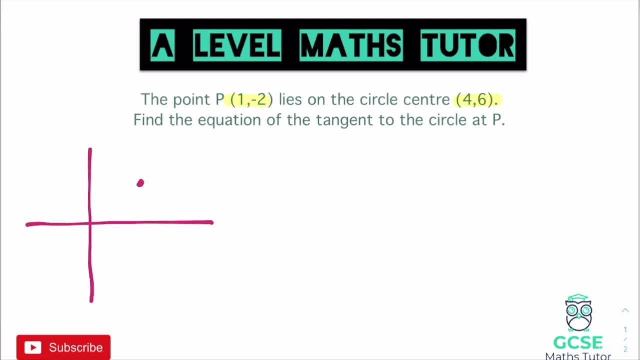 that. that is just there, and there is a point which is across 1 minus 2, let's imagine that's here and obviously you could draw a sketch of the circle Again. it doesn't have to be perfect, but it might help you to visualise it. So we are going to find the gradient of this radius that 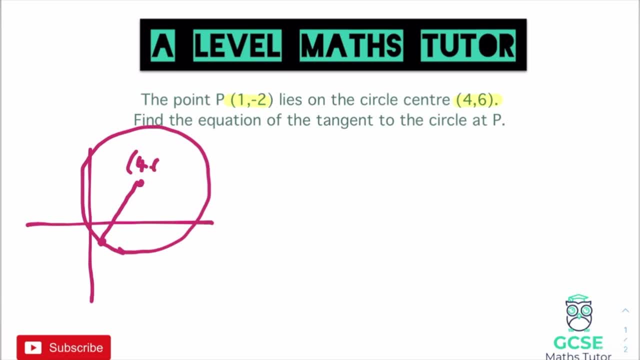 is drawn in and that is between the point 4, 6, and the other coordinate down there, which is 1 minus 2.. So obviously you don't need the actual drawing to do that, because we can just use our y2 minus y1 over x2 minus x1.. So y2 would be 6, take away minus 2 over 4, take away 1.. So 6 take. 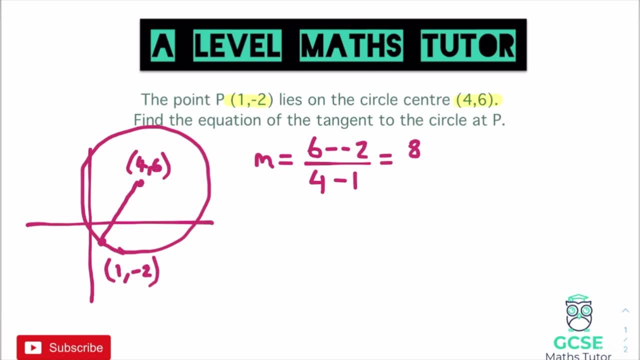 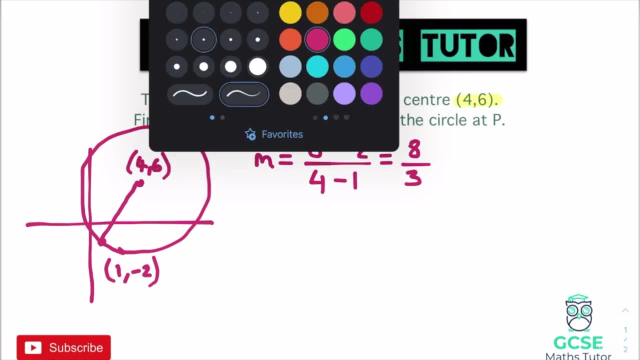 away minus 2 is equal to 8, and 4- take away 1 is equal to 3.. So the gradient of the tangent is 8 over 3.. That means that the gradient of the radius is 8 over 3.. 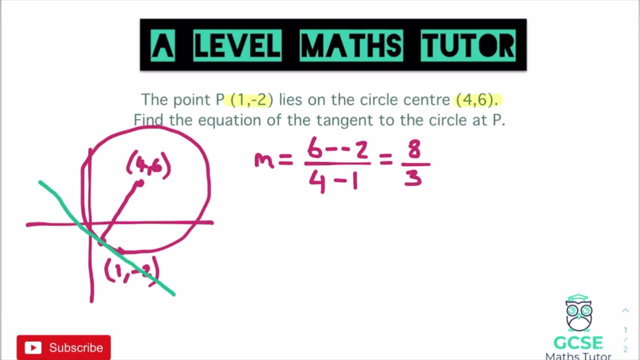 Now we are going to find the gradient of the tangent, because the tangent there is going to have a perpendicular gradient. So we are going to find the perpendicular gradient, which is the negative reciprocal, which is going to be negative 3 over 8.. Now we can take that and we can put it. 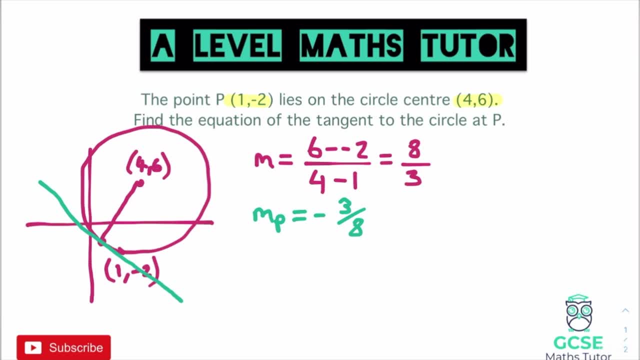 into the equation of the line, given that we know it passes through the point 1 minus 2.. Putting that into the equation of a line, we will have y minus y1, which is y, take away minus 2, which is going to be y plus 2.. So y plus 2 is equal to negative 3 over 8, x minus x1, and x1 is 1,. 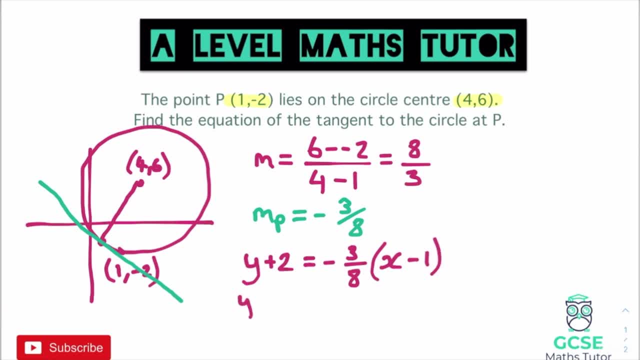 so x minus 1.. We can now expand that so we have y plus 2, which is going to be equal to negative 3 over 8x minus 1.. Times minus 3 over 8 is going to be minus 3 over 8, but it was times a negative, so it would be. 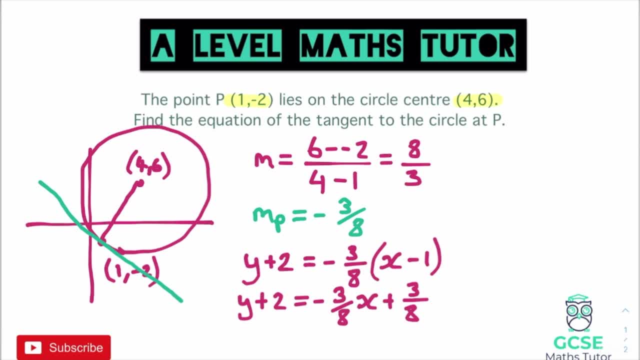 plus 3 over 8.. Now we can take away 2 from both sides, or what we could do here just to make that actually a little bit easier for us is we could just multiply everything by 8 to remove those fractions, and that's fine for us to do So. we would have 8y plus 16 is equal to minus 3x. 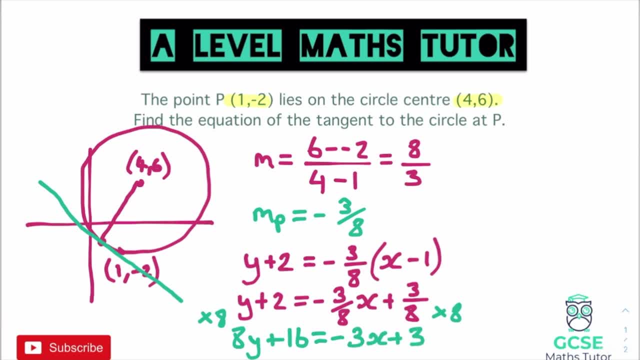 plus 3.. That makes it a lot easier for us to rearrange that and as now, we can just minus 16 from both sides, or we could move everything to one particular side. it doesn't really matter, but if we bring this up here, in fact if we just move everything to the left, then we would have 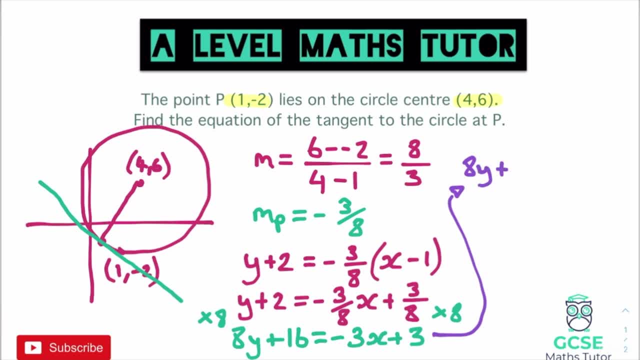 8y plus 3x. when we move that 3x over and also minus the 3 over would give us plus 13, and that is equal to 0.. Of course you could write this as 8y equals. 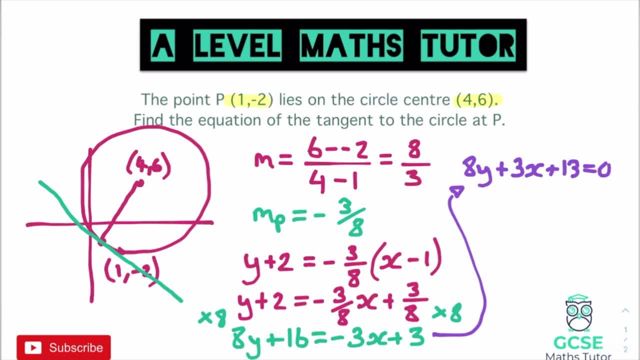 or you could write this as 8y equals, or you could write this as 8y equals, or you could make it y equals if you wanted. the question might ask you to write it in different ways, but it didn't ask us to write it in a particular way, so just having it equal to 0,. 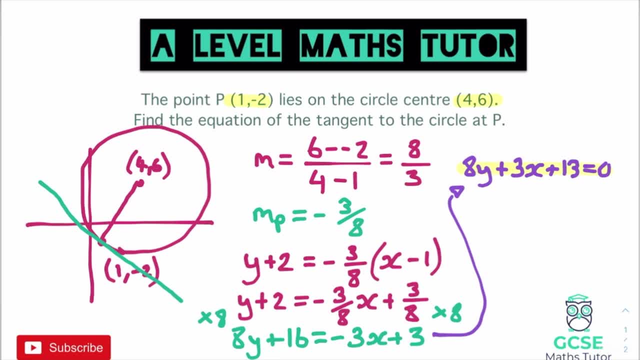 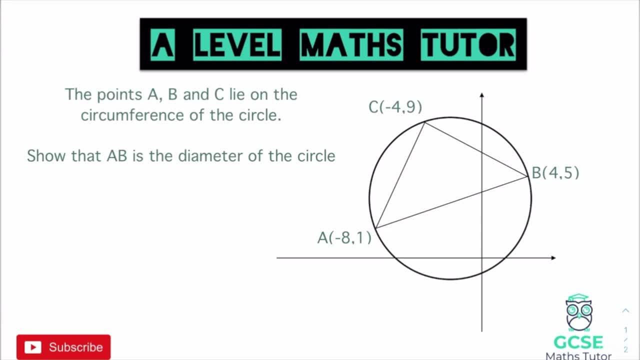 8y plus 3x plus 13 equals 0, is probably the easiest way for us to write that answer. Okay, so when it comes to triangles in circles, there's a couple of different methods that you could use. Now you might be asked to find the centre of the circle. Now this particular question. 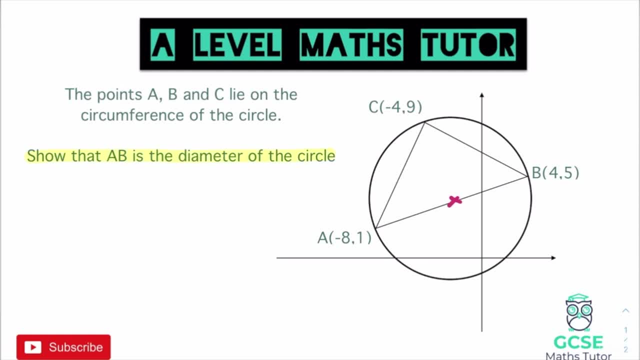 says to show that ab is the diameter of the circle. so of course we could just find the midpoint points of the point a and b. but if it wasn't the diameter of the circle and we were wanting to find the centre, then you could actually use the perpendicular bisectors of the chords. So if we 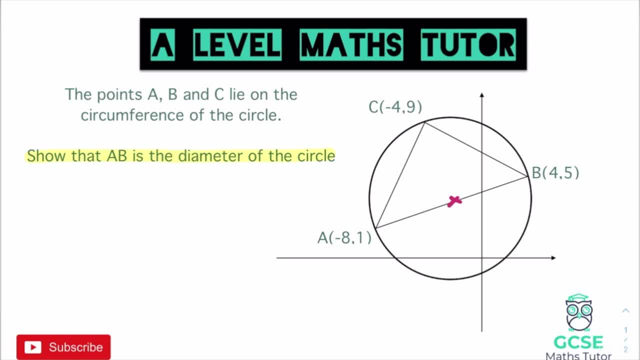 looked at the perpendicular bisector of the chord ac, we would find the midpoint and then find the perpendicular line equation which would go through the circle like this: We could then do the same with cb, finding the midpoint, and again the perpendicular bisector would cross through like: 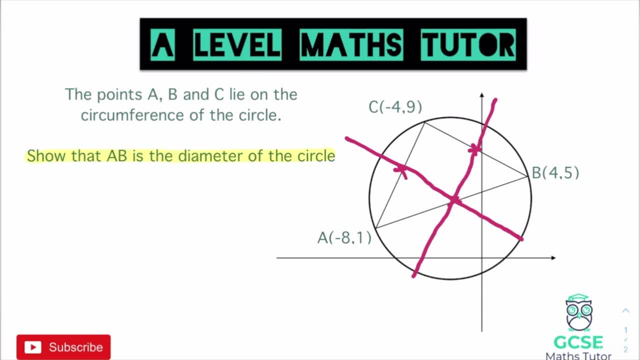 this. Now, those perpendicular bisectors would cross through like this. and if we looked at, the perpendicular bisectors do cross at the centre of the circle. So if you found the equation of those two lines, you could set them equal to each other. And, of course, we've already discussed 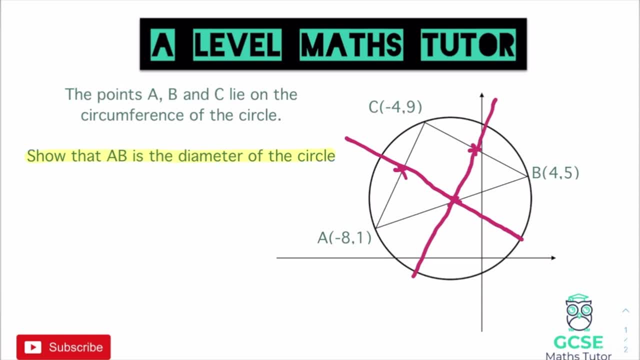 looking at midpoints of lines and perpendicular bisectors, so that additional step there wouldn't be too much work. Now, this particular question is slightly different. It's actually telling us to show that ab is the diameter of the circle. Now, because that is the diameter we know via 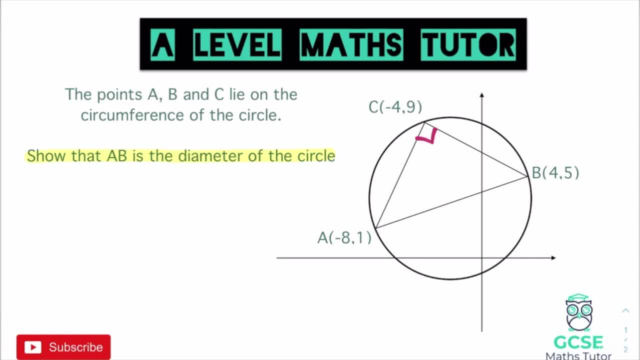 circle theorems that if it is, this angle here must be a right angle and therefore we could use Pythagoras to show this proof. So, in order to use Pythagoras, we would have to find the lengths of these lines, so a to c and c to b. We could then use Pythagoras to show the length that. 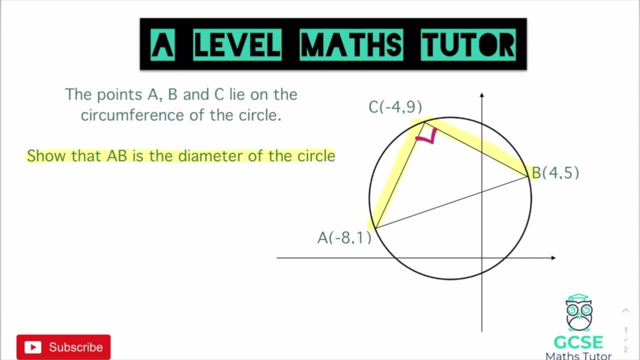 it matches the length of a to b. So if we go about doing that, you can see from a to c the length there goes from minus eight to minus four. Now that is a distance change of four, so we would do four squared. and one to nine is a change of eight. So if we did four squared plus eight squared, 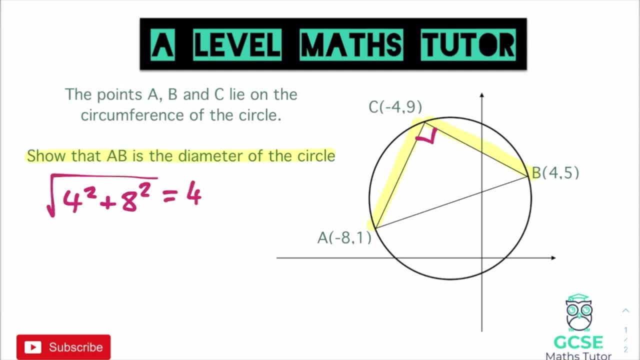 and square rooted our answer. that comes out as four root five. So the length of that line there is four root five. We can do the same from c to b. Now that goes from minus four to four, which is a change of eight, and nine to five is a change of four. So eight squared plus four. 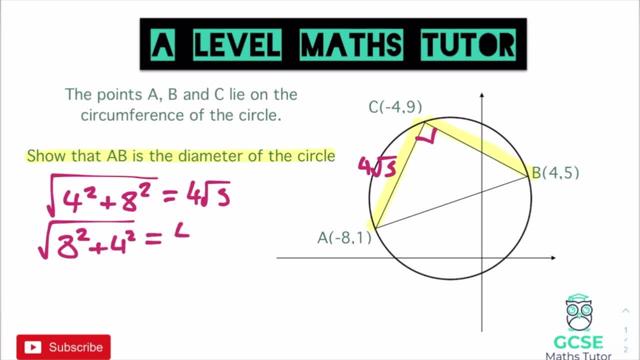 squared for that length. using Pythagoras again would give us four root five. So that length there has a length of four root five which matches the length of a to c. So they are our two lengths and if we do Pythagoras with those two to find the length of the diameter, that should match the